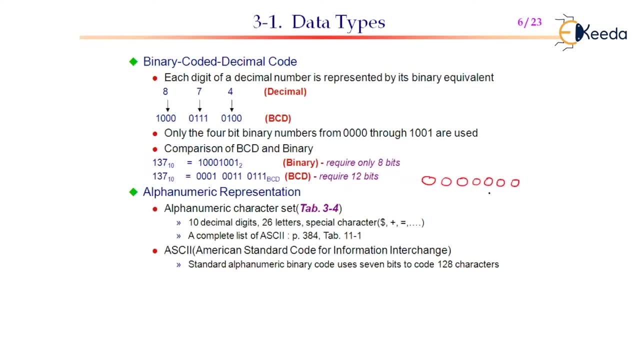 1,, 2,, 3,, 4,, 5,, 6,, 7, as it is shown on the picture. Any ASCII code- either it could be a number or it could be an alphabet or a special character- should be represented by using this 7 digit code. 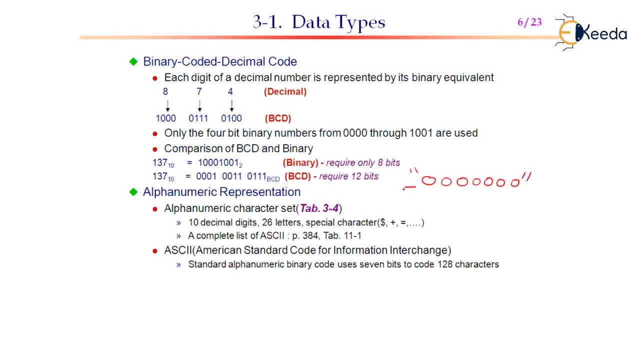 For this, you can clearly understand, we require a byte somewhere in the computer system. That is every time when you type a character that should be transferred to a register which is of 8 bits. Once again, when you try to type something on the keyboard, immediately the 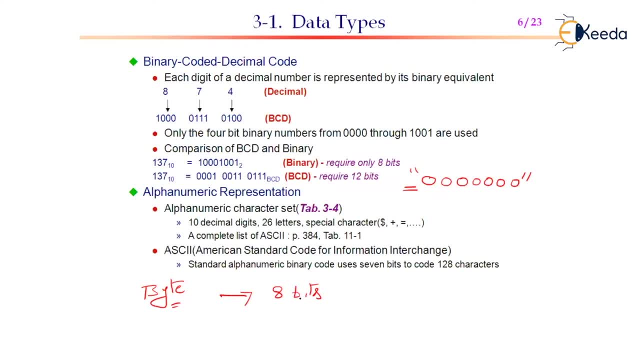 corresponding ASCII code will get generated and immediately it will get transferred to one of the processor's registers, which is of just 8 bits. ASCII code is just 7 bits and we need to obtain the total 8 bits because there is no 7-bit format. 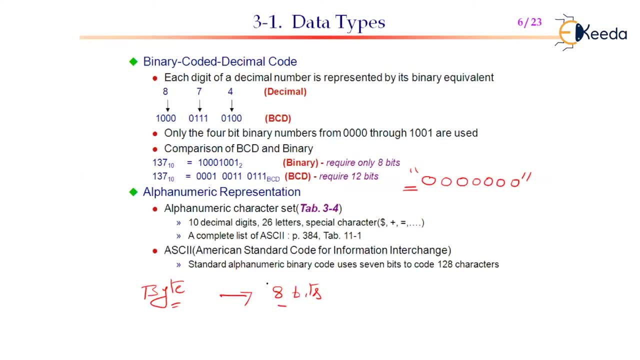 in the computer system, The minimum register size must be 8 bits, because the smallest measurement of storage in any electronic device is 1 byte. So what we would take is we are going to obtain a register which is of 8 bits and in which we will just use the least significant, 7 digits. 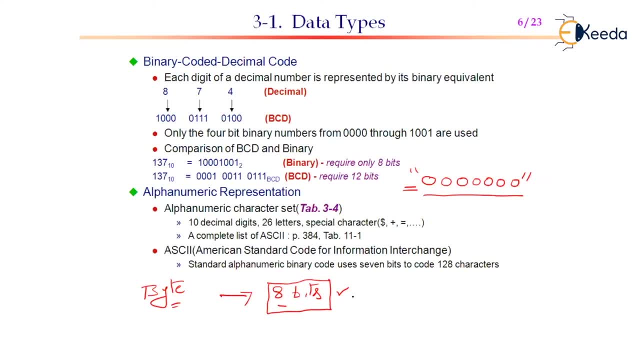 And the most significant bit will be used for some special purposes. We are going to discuss about that register and why the additional digit is going to be used for the other purposes in the upcoming sessions. So for ASCII code, for storing an ASCII code, although it is just seven bits, we do obtain a total of eight bits in the computer. 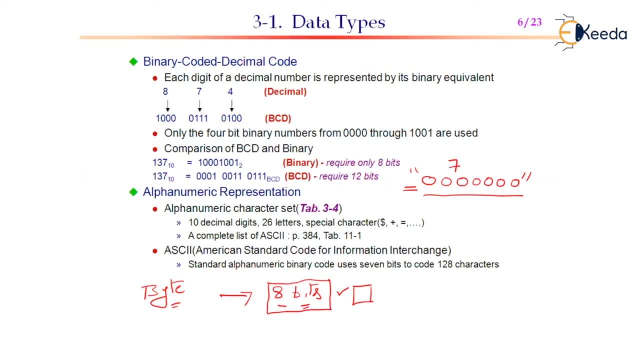 system And now these ASCII code. we do have 10 decimal digits, that is 0 to 9, and 26 alphabets, not only 26,. these 26 will make 52 alphabets up, that is, 26 small letters and 26 capital letters. 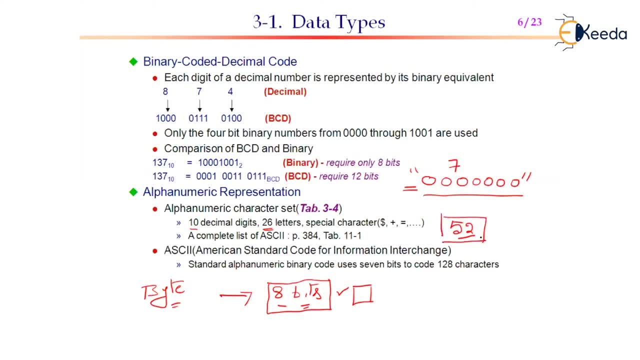 Altogether, we do have a total of 52 alphabets, and in addition to this we have special characters. Every time when you press a key, the corresponding ASCII code will get generated and will get transferred to the processor's register in which it is intended. 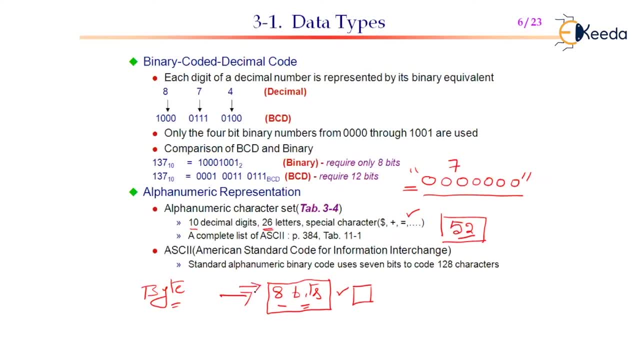 to be transferred. I told you right. there is a register which is going to receive the character that you have generated by using either keyboard or mouse, which is just nothing but an ASCII code. Let me show you a table Here, as you can clearly see. 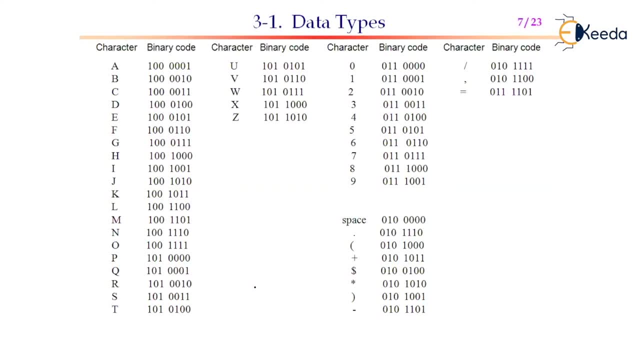 we do have all the alphabets, the capital alphabets, let us say, in addition to the characters and the special characters. Every alphabet when you type- let us say you typed G, G- has a corresponding representation within the ASCII code The moment you press G. 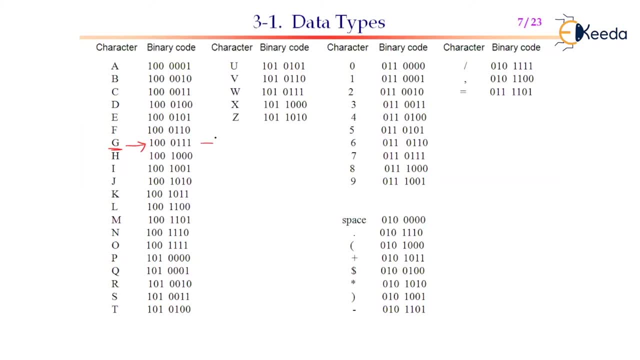 this ASCII code will get generated and will get transferred to the processor's register, followed by the character that you typed. This is a continuous process. as long as you keep up on typing by using the keyboard, The characters will get generated. will get transferred to the 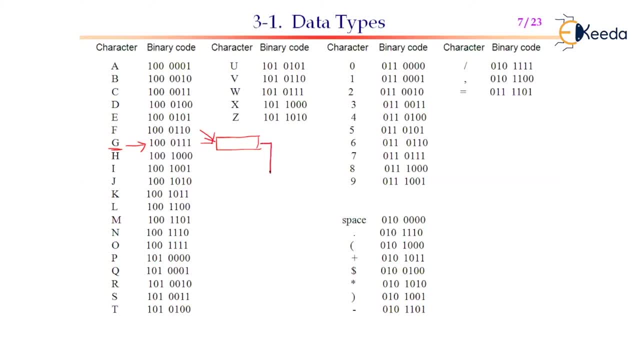 processor's register intermediately. Finally, from that register to the main memory it will get transferred. Let us say this is main memory and this is an intermediate register. Once again, when you type a character, this character will get a corresponding ASCII representation. 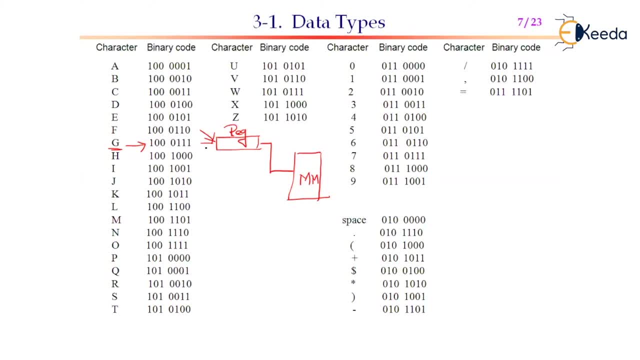 will have a corresponding ASCII representation. That ASCII representation will get transferred to the processor's register. Finally, from the processor's register to the main memory, the typed character will get transferred. Why everything should eventually get transferred to the main memory? The fundamental rule for this is: all the programs are residing in the main memory. 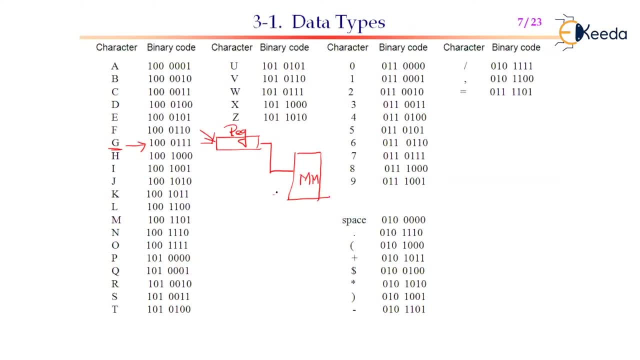 The fundamental logic behind this is: all the programs and the data resides within the main memory. So for that reason, whatever either you give an input or you take an output, the data will get originated and designated in the main memory. The data's final origin or the destination is only the main memory. 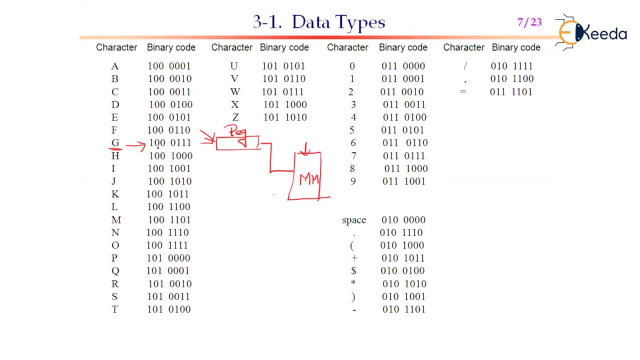 So what initially will happen is, every time when you type a character, there is a processor register which is going to act as a receptionist to receive your data From that register to the main memory. eventually it will get transferred. So this is the complete list of ASCII codes that are going to get generated. 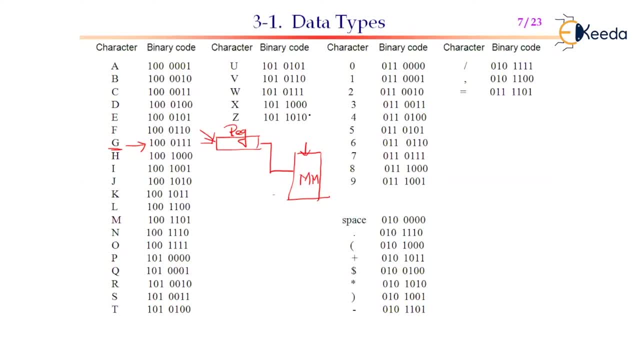 Every time, when you generate them, when you use them, you are going to get an output by using either keyboard or mouse. This is what all about the alphanumeric representation. Similarly, let me tell you- let us say you want to produce an output. 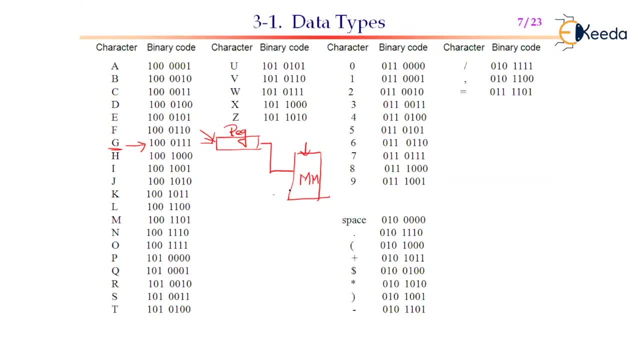 Let us say you just wanted to, you know, print something on the screen. Rather, you just want to take a printout. So, eventually, what is a printer? Printer is also a peripheral device, No matter whichever peripheral device you're using. 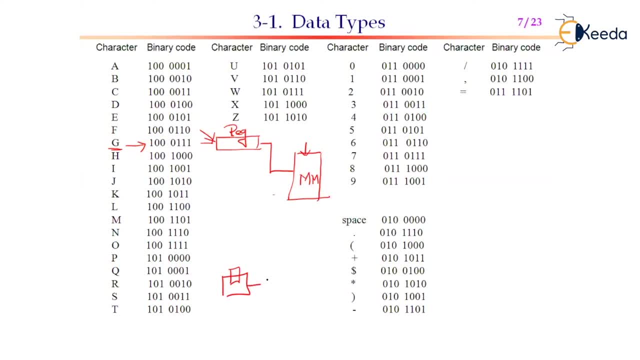 all the peripheral devices will work only under ASCII codes. Let us say there is a character that is needed to be printed on a printer. Now the characters that are stored in the computer system are essentially in the computer understandable format, such as BCD or binary. 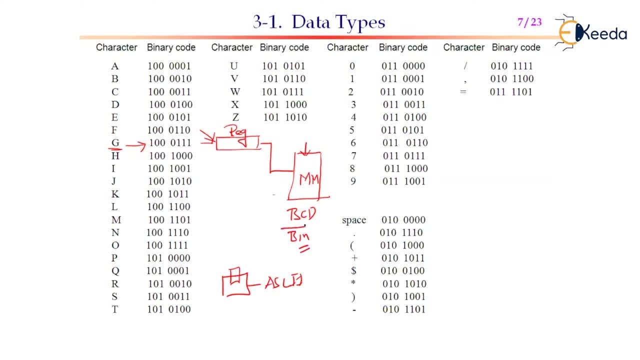 Right Now, if you use a binary format, let us say the computer system is following simply the binary format. If you want to transfer the data to the peripheral device, again from binary format to ASCII format, the character will get transferred, The character will get translated. 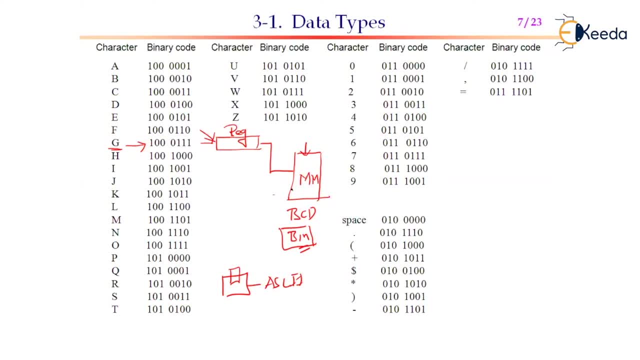 After which the translated character will get transferred from main memory to a processor's register which acts as the intermediate register to communicate with the peripheral devices. for the outputs, For the inputs, we do have a special register. For the output also, similarly, we do have another register. 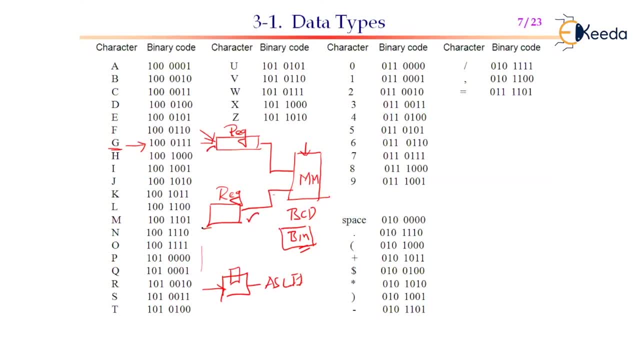 which will initially take the value from the main memory. Finally, it outputs to the peripheral device. This is how it is going to happen every time when you either are going to give the input or take the output from the computer system. And once again, you just need to understand. 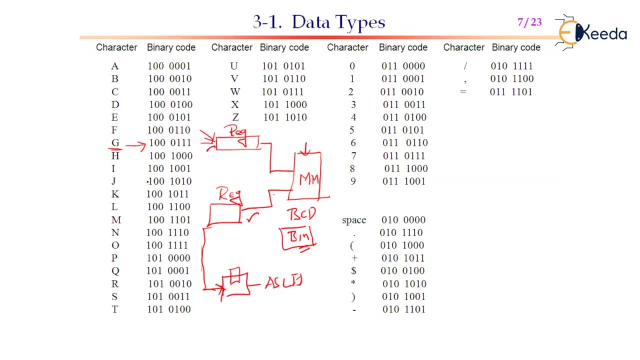 regardless of the computer understandable format, all the peripheral devices just uses the ASCII code. Eventually these codes will have to get translated to the computer understandable data formats. the moment they are getting transferred to the computer system: ASCII to binary. binary to ASCII. 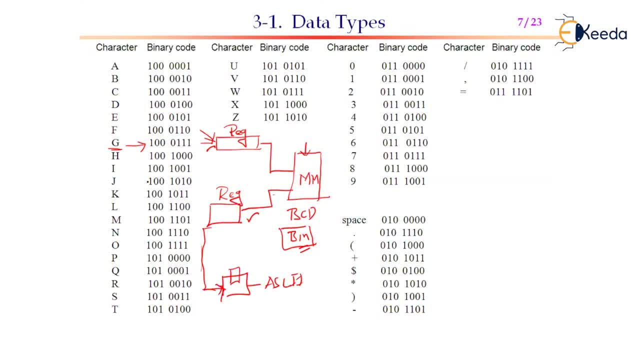 Either you give the input or taking the output. This translation is actually required, Thank you.